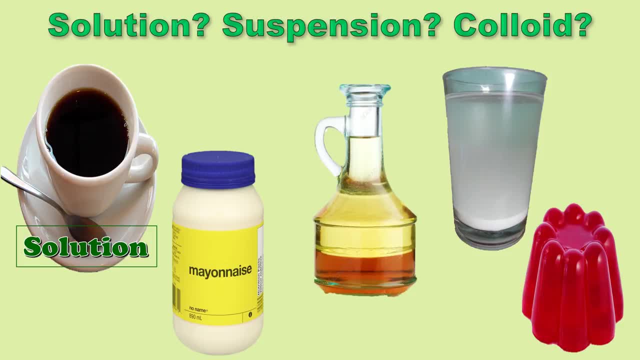 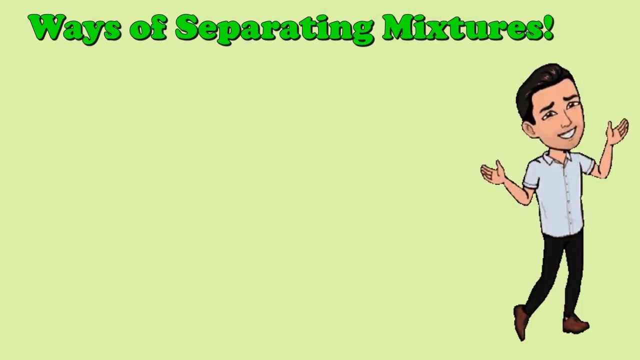 about mayonnaise? Very good, it's a colloid. How about mixture of vinegar and cooking oil? Correct, it's a suspension. How about mixture of flour and water? You're right, it's a suspension. How about gelatin? Yes, gelatin is a colloid. Today, our topic is all about ways of separating. 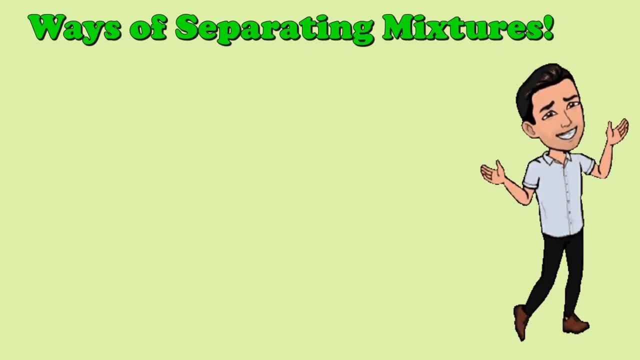 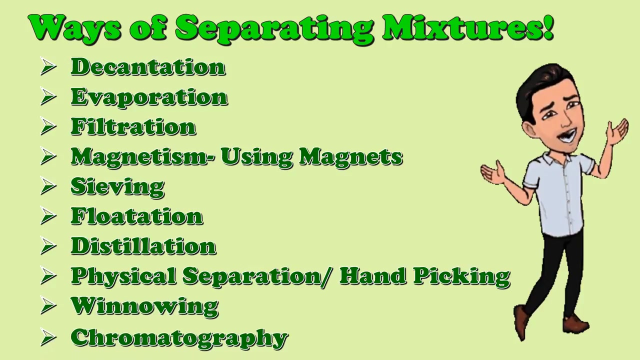 mixture. There are different ways in separating mixture. We have the following: Decantation, evaporation, filtration, magnetism or using magnets sieving flutation, distillation, physical separation or hand-picking, winnowing and chromatography. 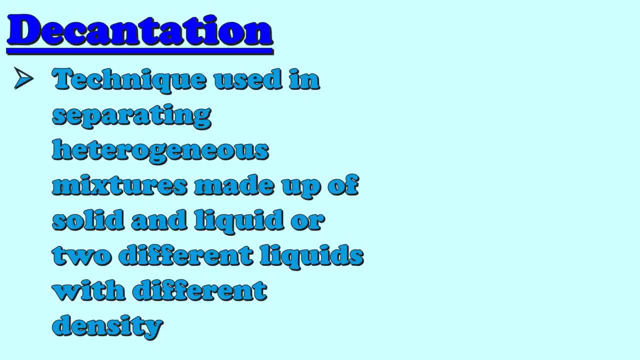 Let us first discuss what decantation is. Decantation is a technique used to separate mixture. Decantation is used in separating heterogeneous mixtures made up of solid and liquid or two liquids with different density. In the process of decantation, the mixture is left undistributed. 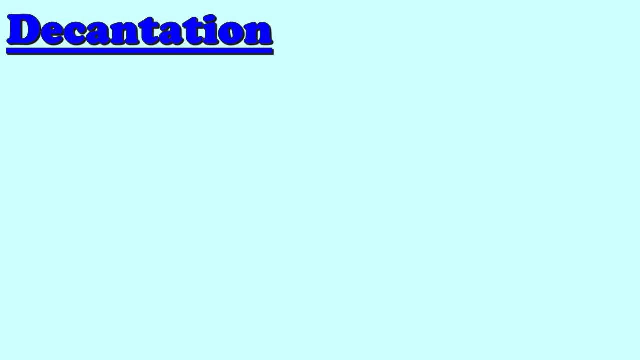 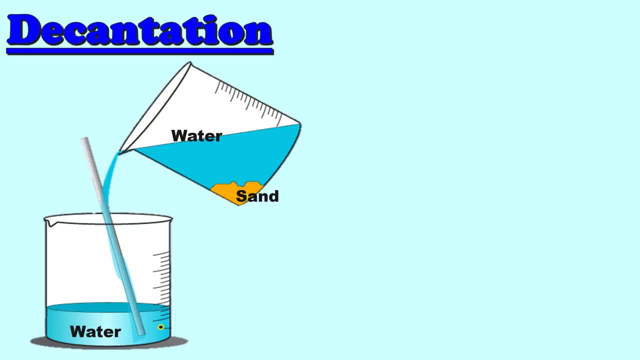 Once the sand is settled at the bottom of the container, you can easily separate water from it by powering to the other container is another example that can be separated through. decantation is a mixture of oil and water Because They have different density. Oil can be separated by scooping using a spoon. 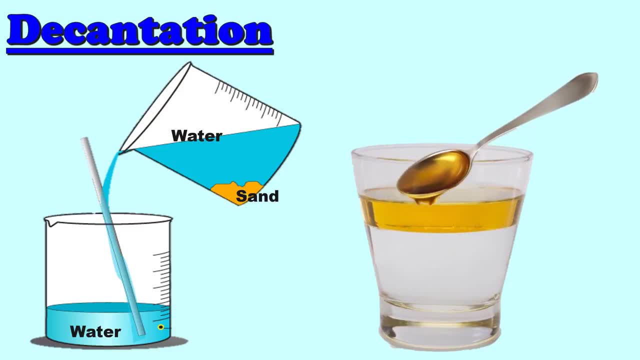 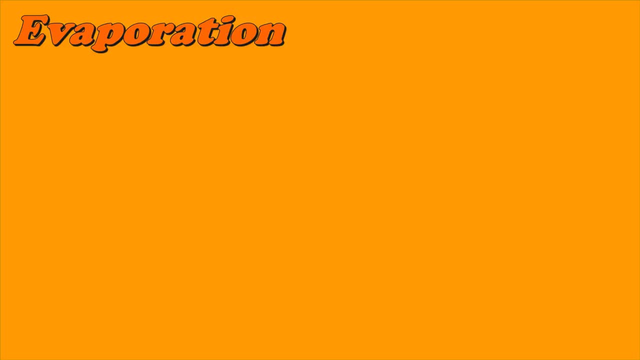 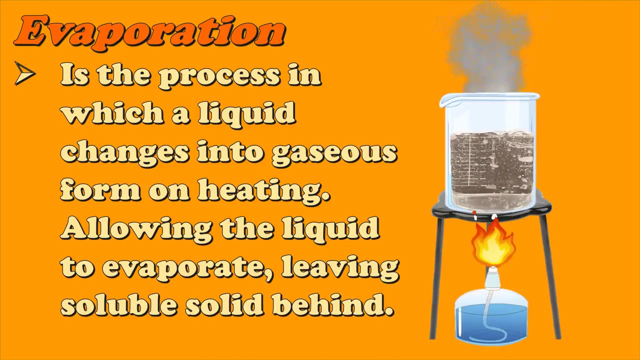 How to separate sand and water. How to separate sand and water. Another way of separating sand and water is by savory evaporating mixture, is what we called evaporation. It is the process in which a liquid changes into gaseous form on heating, allowing the liquid to evaporate, leaving the soluble solid. 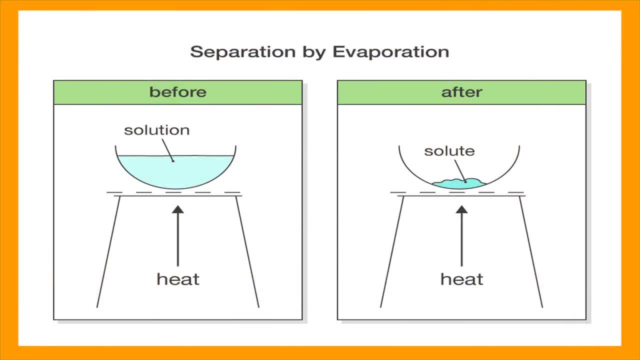 behind This method also produce salt by evaporating sea water under the sun. When a salt solution is heated, water evaporates and turns into gas, or what we called water vapor, and salt remains in the container. The remaining residue is the solute Grains. of salt remains in the 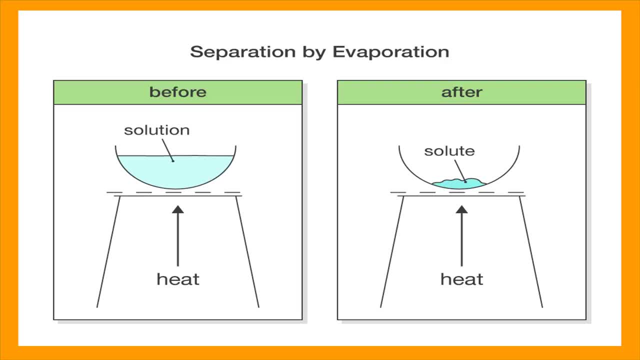 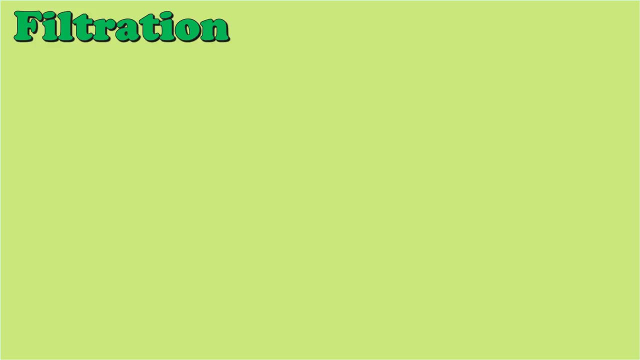 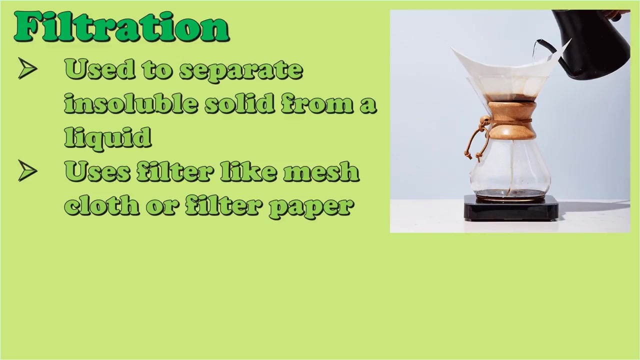 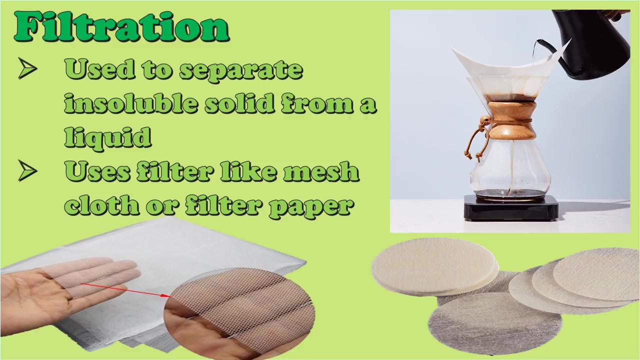 container as the liquid evaporates. Remember that in evaporation only the solute is recovered, not dissolved. Another technique to separate mixture is what we called filtration. filtration is used to separate insoluble solid from a liquid. it uses a filter like mesh cloth or filter paper at this. 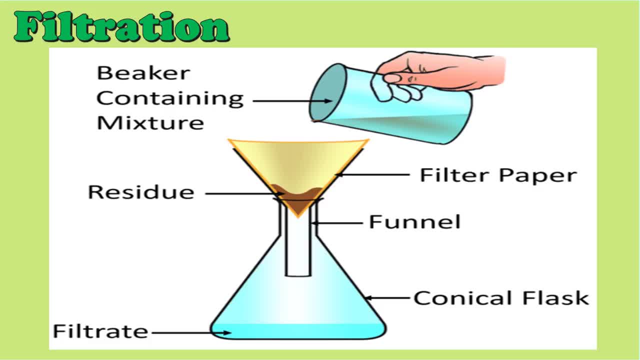 illustration: a mixture of liquid and tiny particles of solid which have not been dissolved can be separated through filtration. a filter paper is used to separate the suspended particles from the liquid. it has a tiny pores that allow the liquid part of the mixture to pass through it. the solid particles that 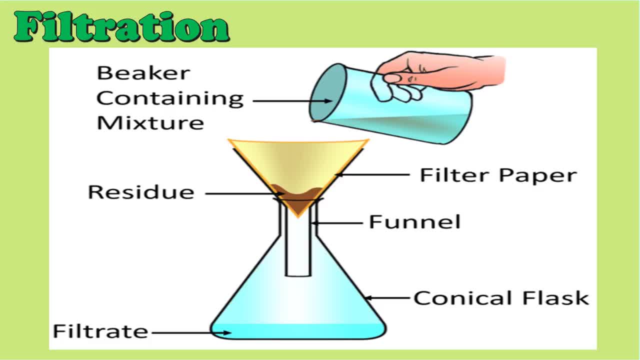 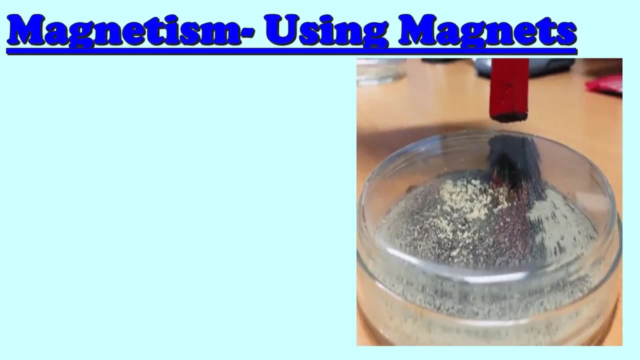 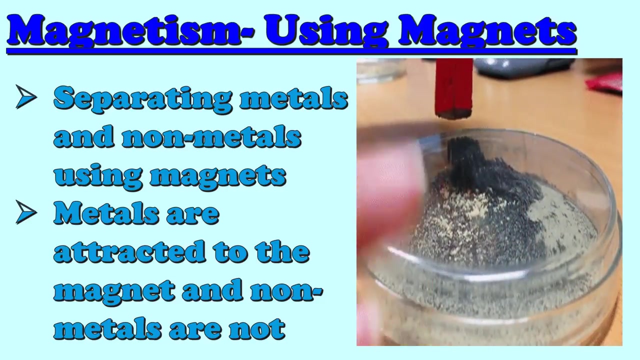 are left behind are called residue, while the liquid that passes through the filter paper is called filtering. a clean piece of cloth can also be used if the filter paper is used to filter the liquid out of the mixture. the filter paper is not available. magnetism or separating mixture using magnets. it is used to 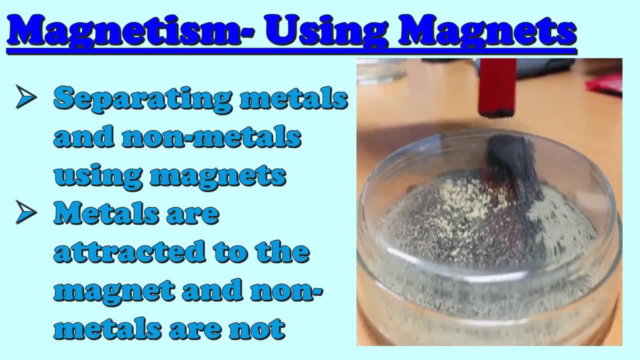 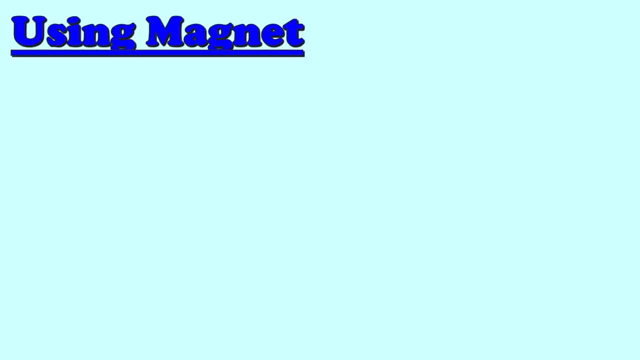 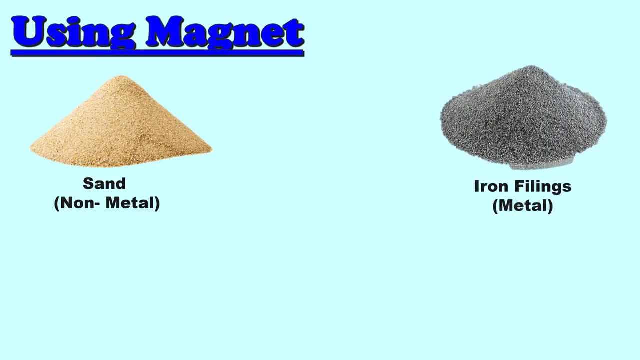 separate metals and nonmetals using magnets. metals are attracted to the magnet and nonmetals are not. one example of a mixture that can be separated using magnet is a mixture of sand and iron fillings. when iron fillings are mixed with sand, they form a mixture, but they 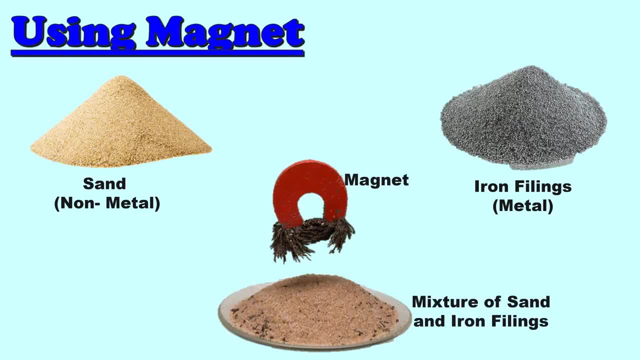 keep their original properties. the iron remains magnetic, while the sand stays non-magnetic. looking at the mixture, it is pretty visible that the dark brown iron speckles the yellow sand. when a piece of magnet is placed over the mixture and move about, the iron, iron fillings are attracted to the magnet, leaving the sound on the disc. 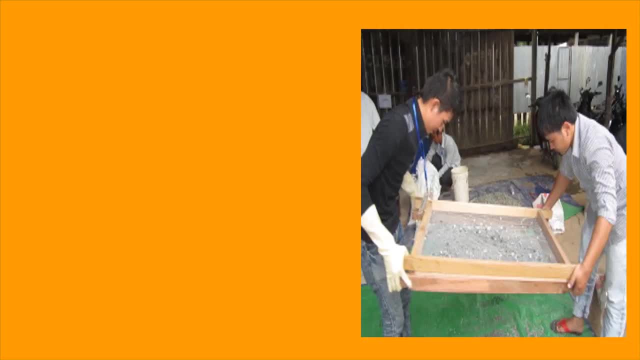 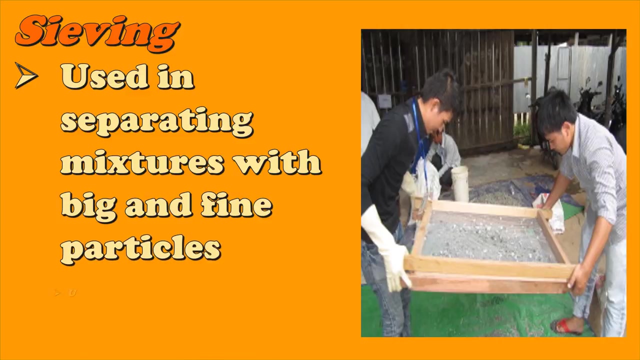 Have you seen the same scenario in your community or in a construction site? This picture shows us another way of separating mixture, known as sieving or sifting. It is a method used in separating mixture with big and tiny particles using a strainer or a big screen. 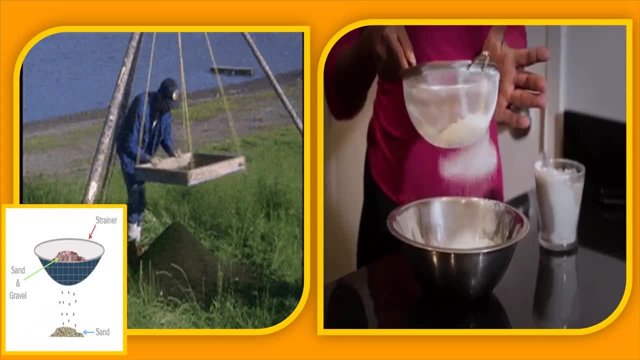 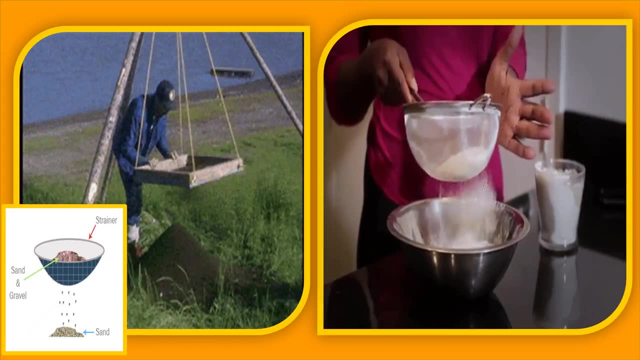 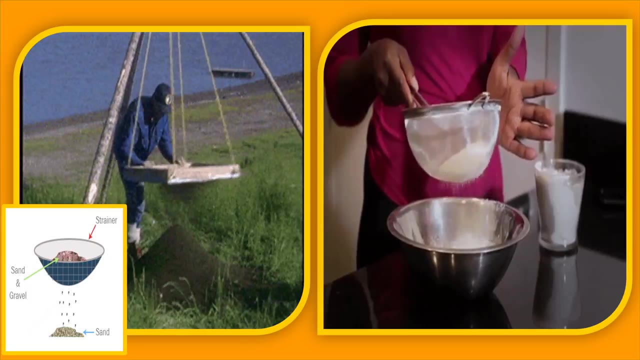 Here are some examples of mixture that can be separated through sieving. Separating the sand from gravel through sifting The strainer allows only the fine particles through it and prevents the larger ones. The sieving technique is used in separating fine sand from rocks in the mixture of gravel. 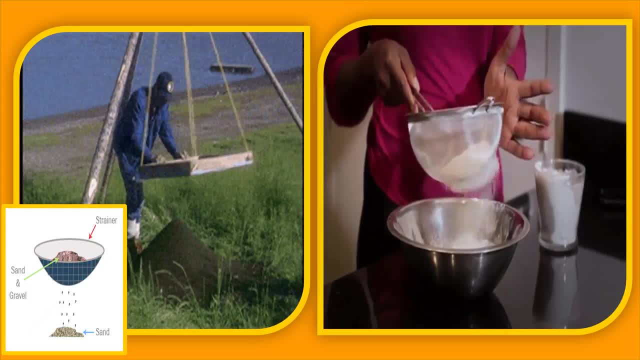 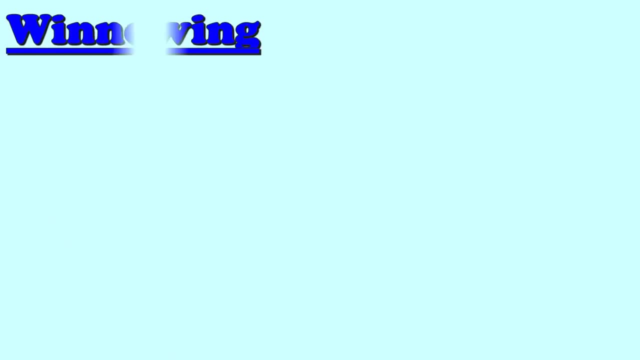 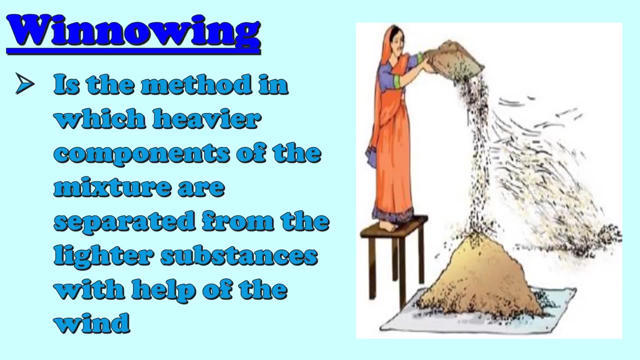 and sand And, of course, separating large size of flour using a strainer. We have winnowing. It is the method in which heavier components of the mixture are separated from the lighter substances with the help of the wind, And the instrument used in winnowing is what we call winnower. 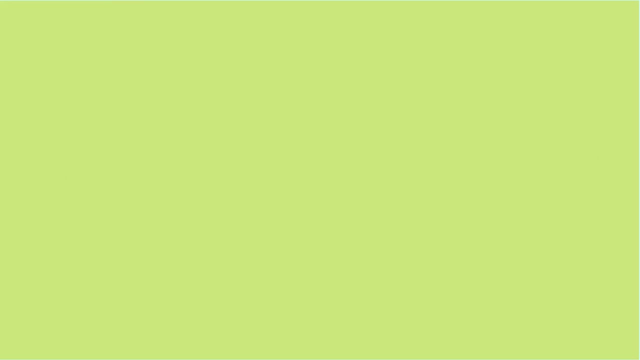 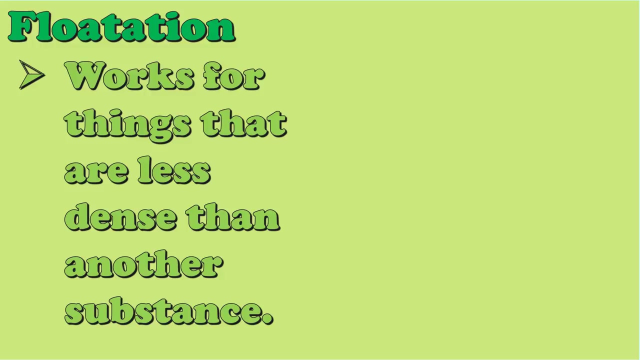 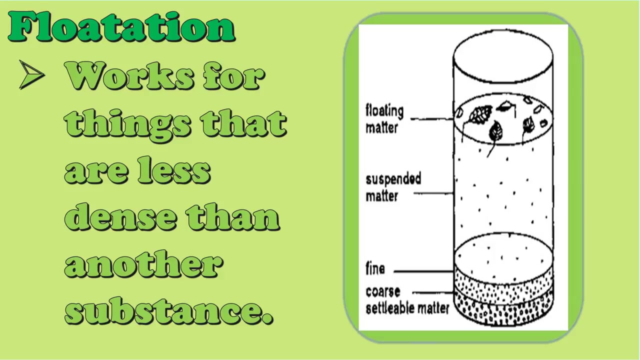 Another way of separating mixture is known as flotation. It works for the things that are less dense than another subsets, Like leaves, that would float in water. When it happens that the water you are about to use in washing your hands has floating particles like leaves, you can easily separate the particles because they are floating. 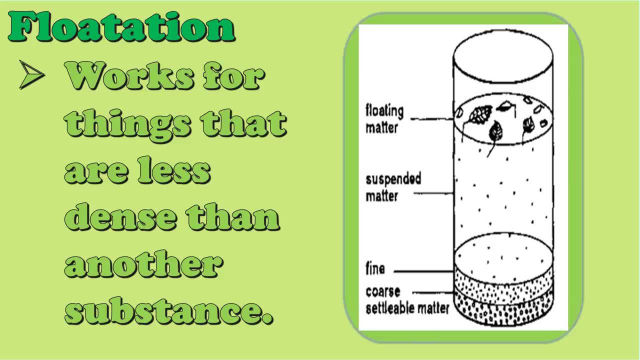 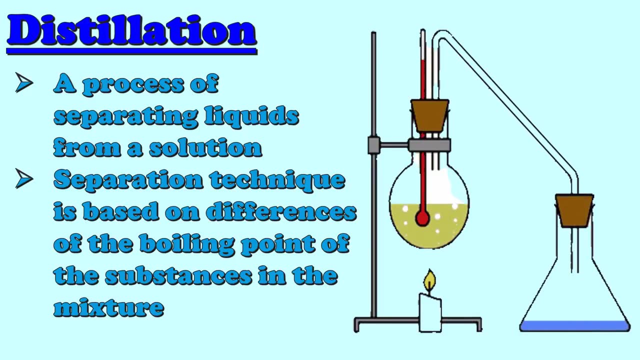 When you are washing the rice that you are about to cook, there are smaller particles of rice bran floating in the water. You can easily separate the floating particles. We have distillation. Distillation is the process of separating liquids from a solution. The separation technique is based on the differences of the boiling point of the substances in 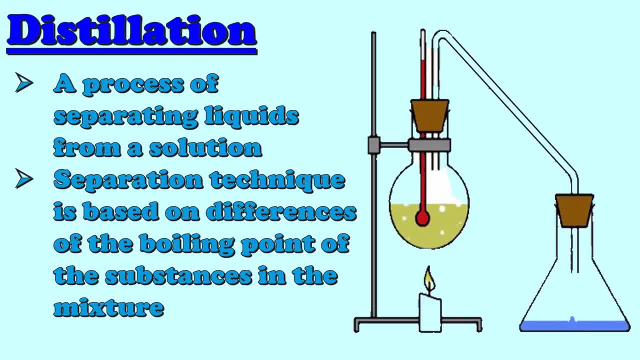 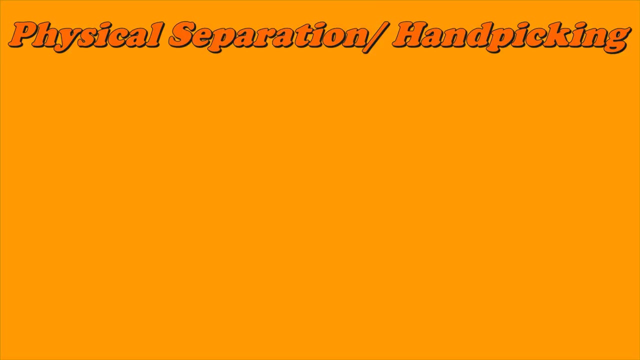 the mixture. In distillation, a mixture is heated. The substance with the lowest boiling point boils to vapor And condenses to liquid. It is collected as distilled water. Most homogeneous solution can be separated by distillation. This, their technique, is what we call physical separation or hand-picking. 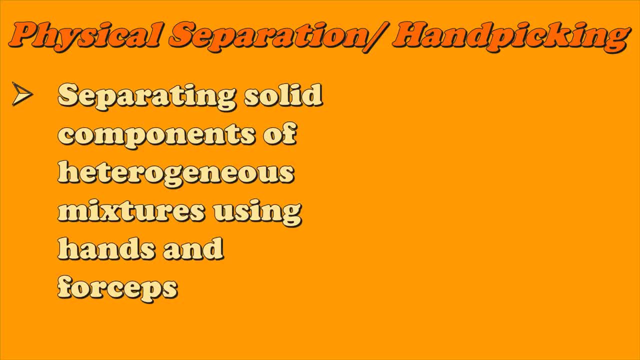 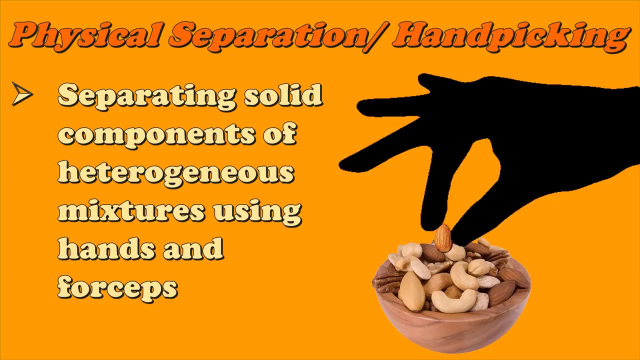 It is a technique used in separating solid components of a heterogeneous mixture. The components of a mixture should be big enough to be seen and dreied in the mixing picked by the hands or forceps. When you separate nuts in a mix nuts, you can separate the components through physical manipulation or by the use of your hands. 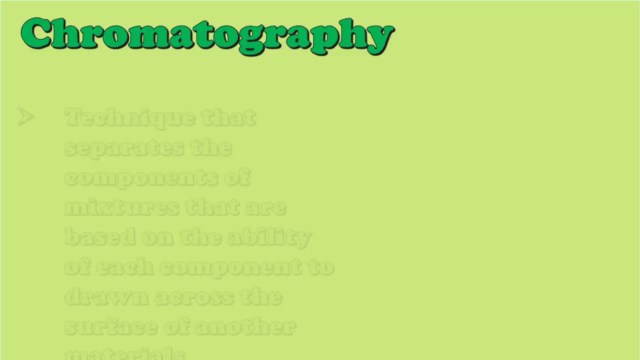 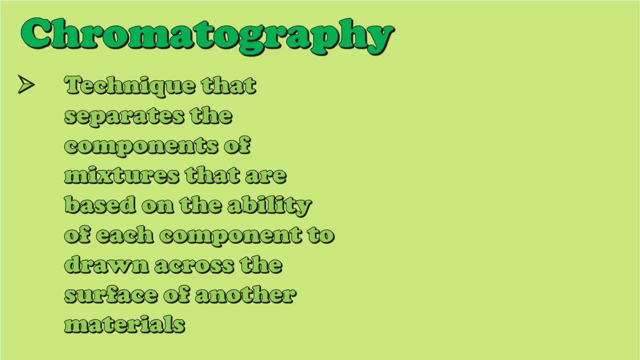 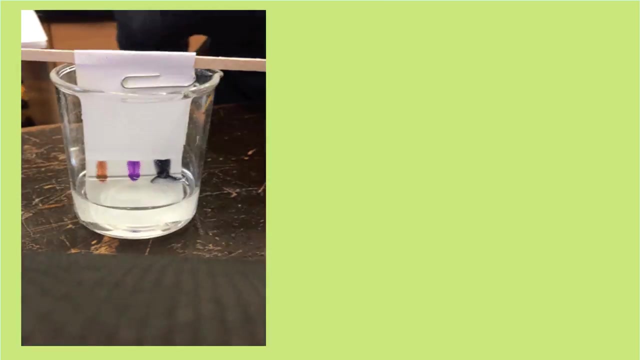 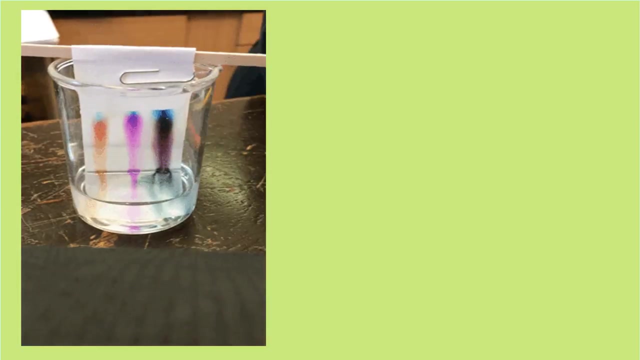 Last technique is what we call chromatography. It is a technique that separates the components of mixture that are based on the ability of each component to drone across a surface of another material. During the separation, the various components or materials spread in different speed. Chromatography is good in separating dissolved substances that have 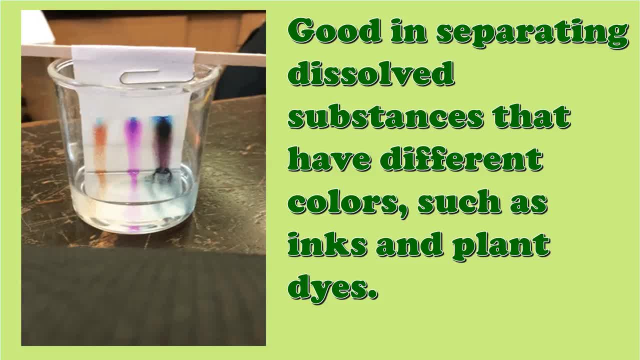 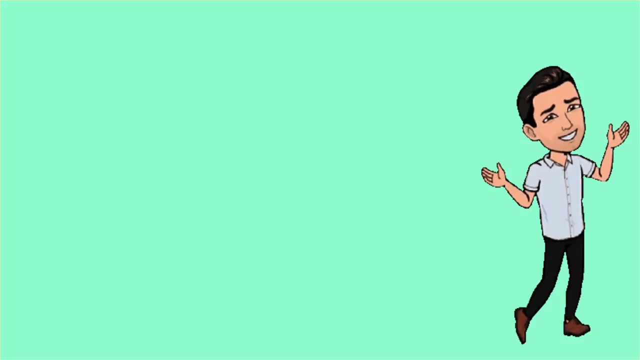 different colors, such as ink and plant dyes. Chromatography works in separating dyes because some of the colored substances dissolve in liquid better than others, So they travel further up the paper. Now can you identify the different ways or techniques in separating mixture? 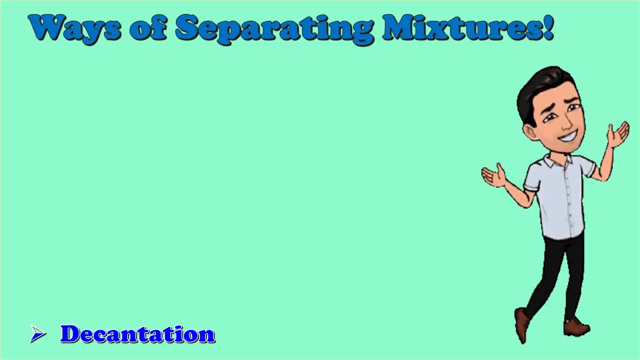 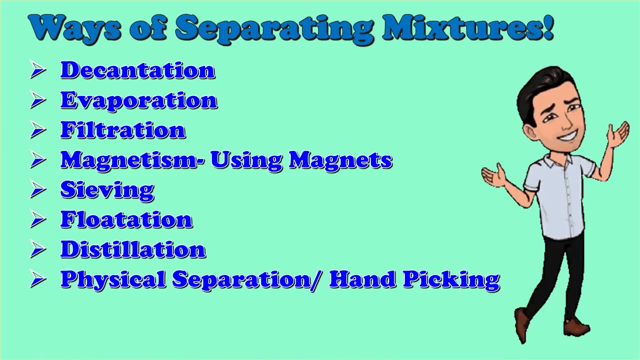 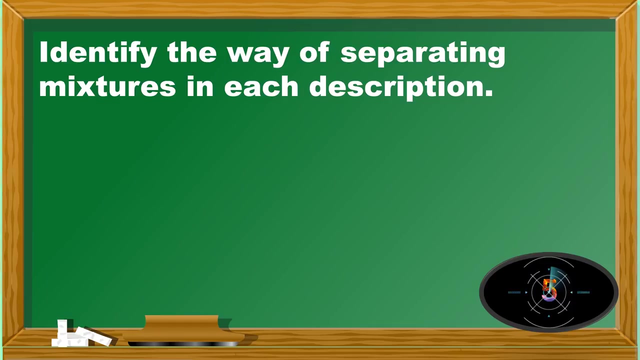 Very good, Let's go. We have Decantation, Evaporation, Filtration, Magnetism or using magnets, Sieving, Rotation, Destillation, Physical separation or hand picking, Winnowing Chromatography. Now let's find out if you learned something from our discussion. 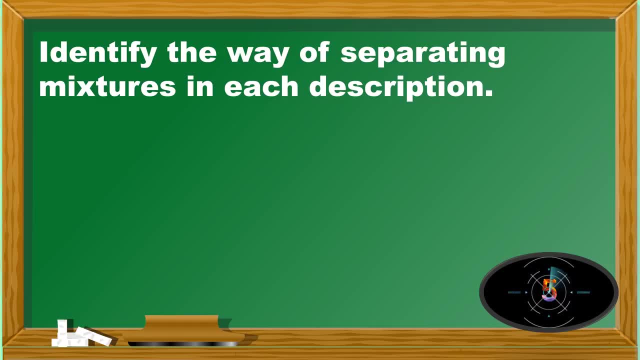 Let's have a quiz: Identify the way of separating mixture in each description. You have 5 seconds to answer each question. Number 1.: Use to separate mixture with big and fine particles using a strainer. Go, The correct answer is sieving Correct.